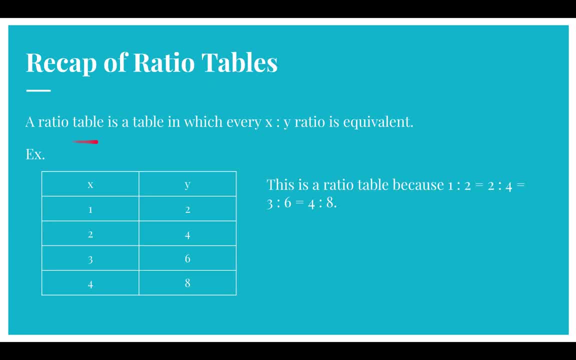 So let's recap ratio tables. A ratio table is a table in which every x to y ratio is equivalent. And we have an example of a ratio table right here, And we know that this is a ratio table because 1 to 2 is equal to 2 to 4, which is equal to 3 to 6, which is equal to 4 to 8.. 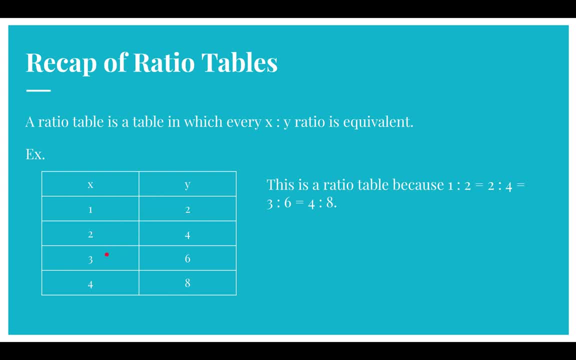 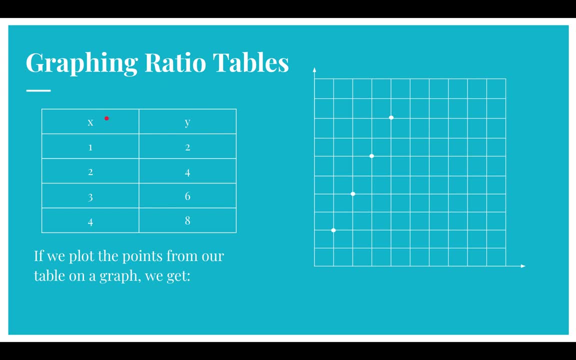 Every single x to y ratio we have is equivalent. So now let's learn how to graph ratio tables. So from this x and y table, we have four points. We have 1,, 2,, 2,, 4,, 3, 6, and 4, 8.. 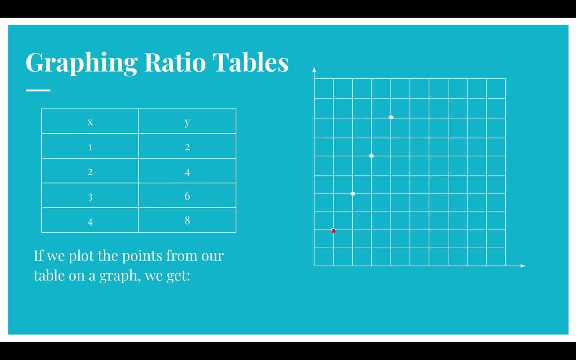 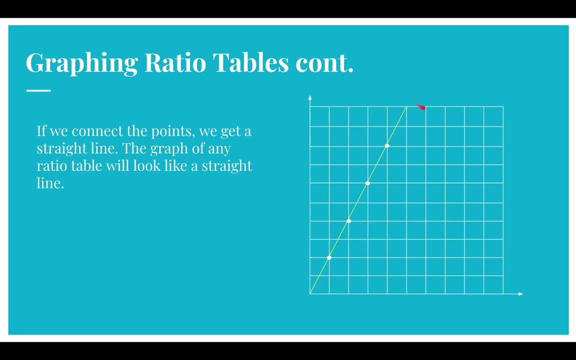 So let's plot these. We get 1, 2.. 1, 2, 4,, 3, 6, and 4, 8.. And if we connect these points, we get a straight line. The graph of any ratio table will look like a straight line, no matter what the ratio is. 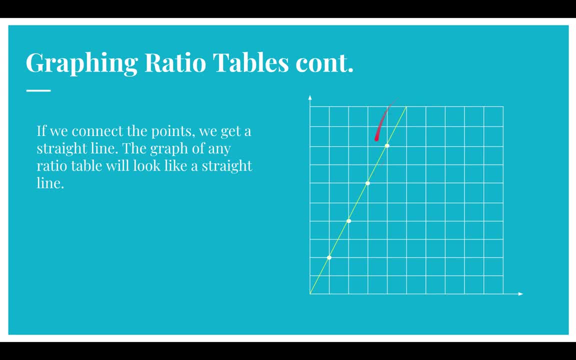 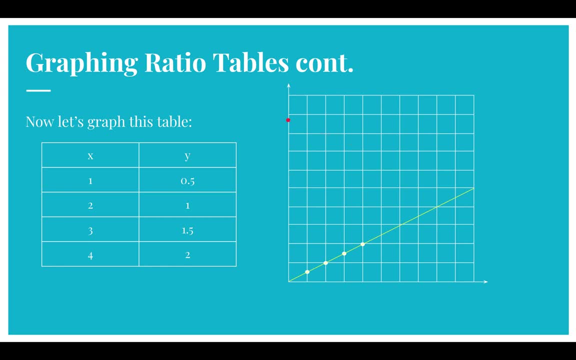 If you're graphing a ratio table and you don't get a straight line, you've either graphed it incorrectly or you don't have a ratio table at all. Let's do one more example. Let's graph this table now. We have four points again. 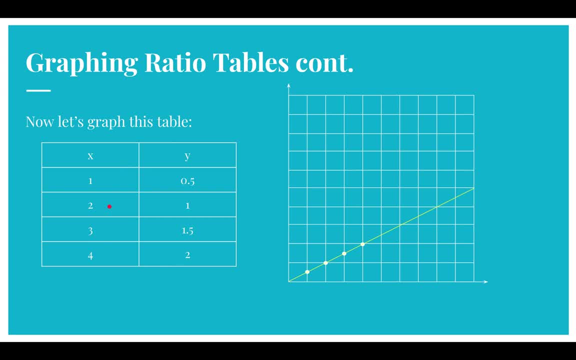 We have 1, 0.5,, 2,, 1,, 3, 1.5, and 4, 2.. So if we plot this, we get: this is 1.5,, this is 2, 1,, this is 3, 1.5, and 4, 2.. And notice that these also 1.5,, 2,, 1,, 3,, 1.5, and 4, 2.. And notice that these also 1.5,, 2,, 1,, 3,, 1.5, and 4, 2.. 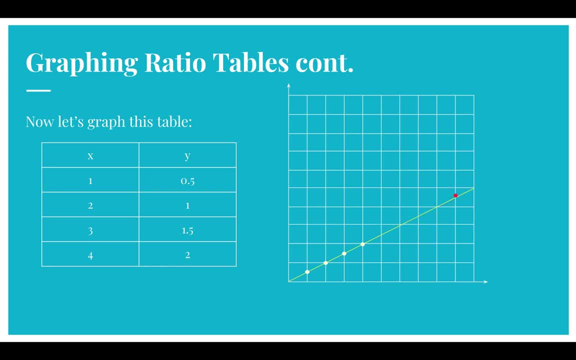 1.5,, 2,, 1,, 3,, 1.5, and 4, 2.. 1.5,, 2, 1.5, and 4, 2.. also form a straight line, just like any other ratio table will. So now let's. 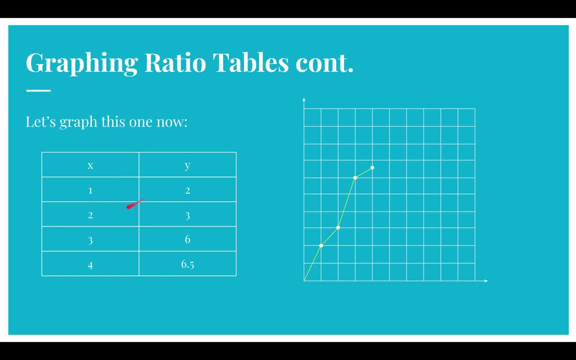 graph this table Once again. we have four points. We have 1, 2,, 2,, 3,, 3, 6, and 4, 6.5.. So we have 1,, 2,, 2,, 3,, 3,, 6, and 4, 6.5.. And notice that these points do not create a. 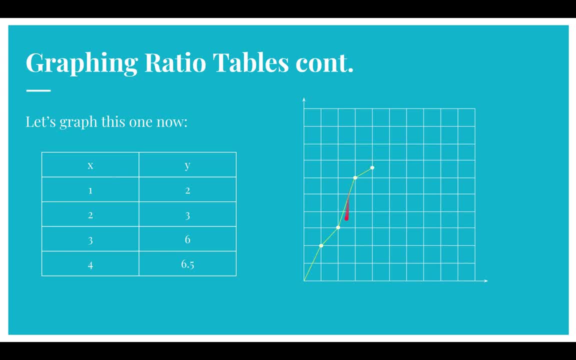 straight line. We have more of a jagged line that connects every point together, And that is because this is not a ratio. table 1 to 2 is not equal to 2 to 3, and that's not equal to 3 to 6, or 4 to 6.5.. None of these ratios are equivalent to each other, which is why 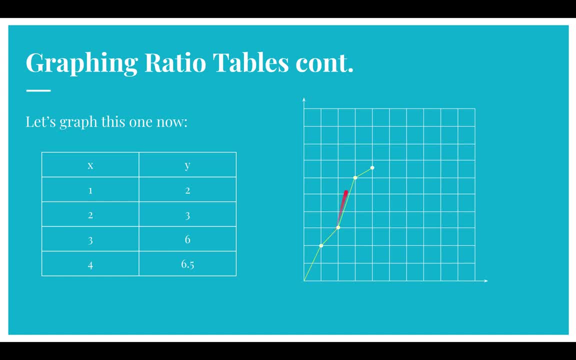 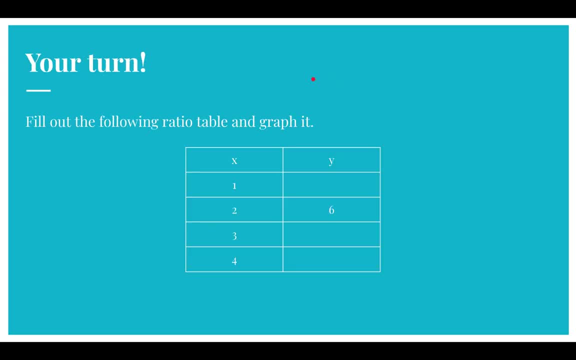 we don't have a ratio table, which is why we don't have a straight line. Instead, we have more of a jagged figure here. Now it's your turn. Pause the video and answer the question. Do you have your answer yet? 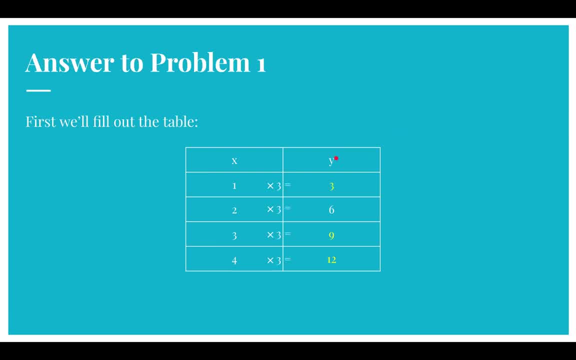 Let's go over it now. So the only y value we're given is 6.. And we ask ourselves: what do we multiply 2 by to get 6?? And if we ask ourselves that, the answer would be 3.. So 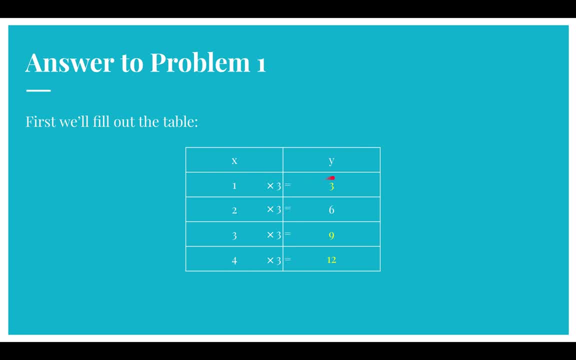 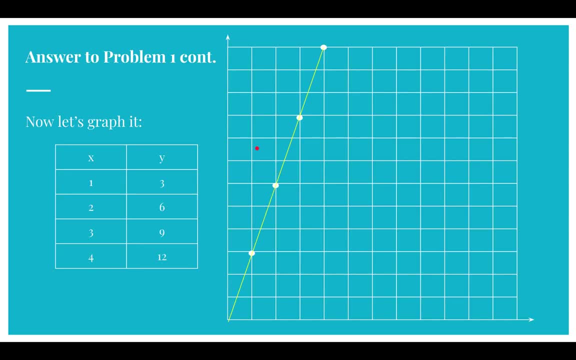 we'll multiply every other x value by 3.. And our missing values are 3,, 9, and 12.. And now let's graph it. So we have our four points, We have 1,, 3,, 2,, 6,, 3,, 9, and 4, 12.. And here we have 1,, 3,, 2,, 6,, 3,, 9, and 4,. 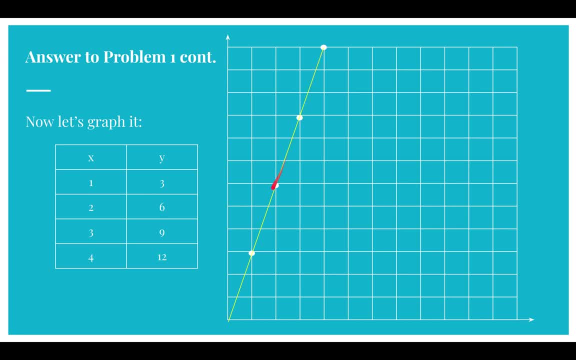 12. And once again, you'll notice that this forms a straight line, if done properly, because we have a straight line. And we have a straight line if done properly because we have a overriding equation of eight. We have 1,, 3,, 2,, 6,, 3,, 9, and 4, 12. And we have a straight. 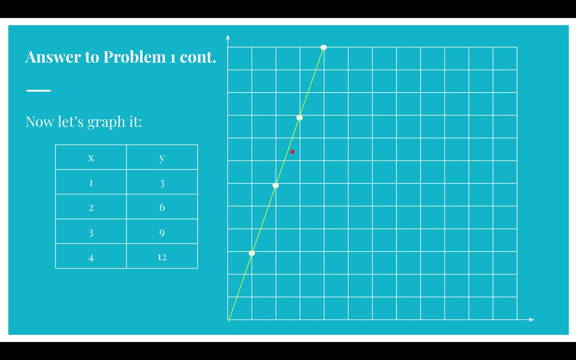 line, if done properly, because we have a straight line. because we have a straight line, So we have 1,, 3,, 2,, 6,, 3,, 9, and 4, 12.. And here we have 1,, 3,, 2,, 6,, 3,, 9, and 4, 12..